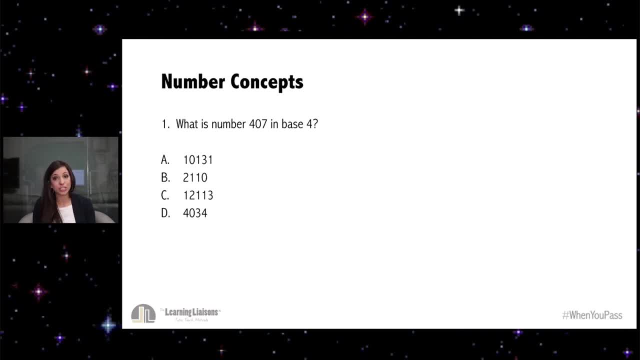 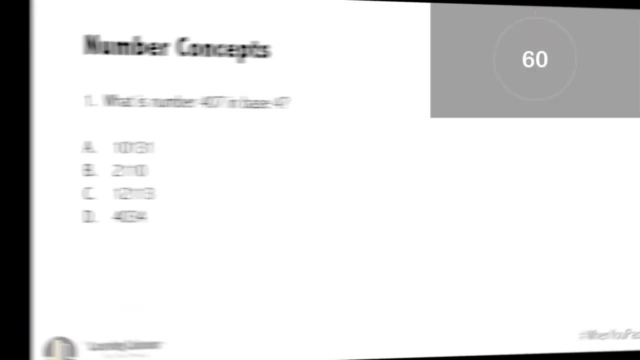 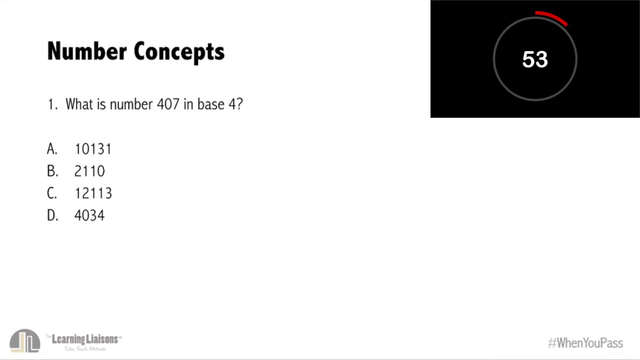 one, one, zero C. one, two. one one three, D four, zero, three, four. You have 60 seconds. Go for it. One, two, three, four. What's the upper delay ratio? 0, 0,wash mix. 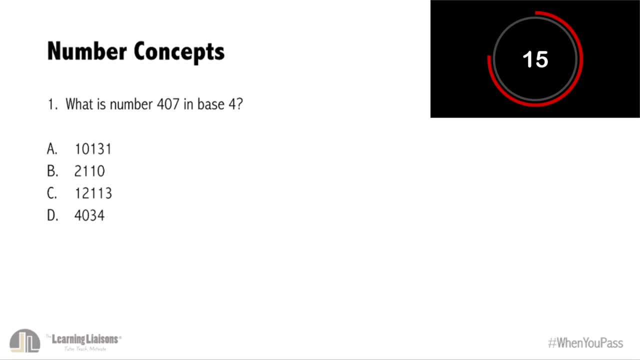 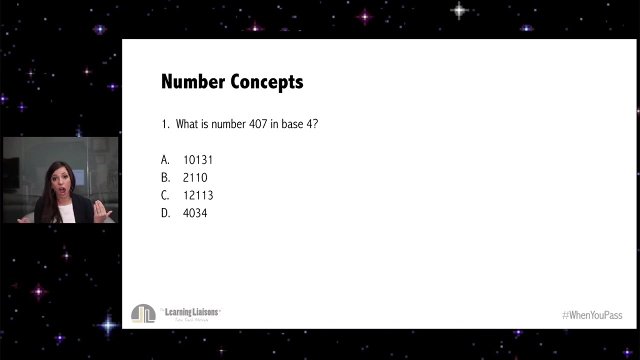 Win. What's the top delay? 3,2,, 0,1-1,, fights, burns, Dansster, Dancer, Legislation, Administrators, Disclosure, Foreman: All right, Base 4 is kind of an abstract concept for most of us. All of our numbers are in. 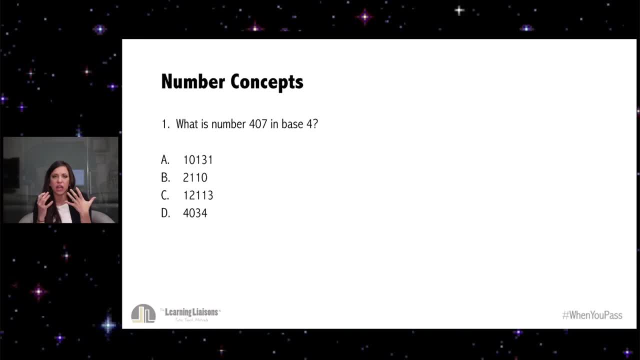 base 10.. So to operate in base 4 is a very odd concept for most of us. In order to figure out what the number is represented in base 4, or any base for that matter- we have to divide that number by the base that we're looking for. So if they ask for base 6, we 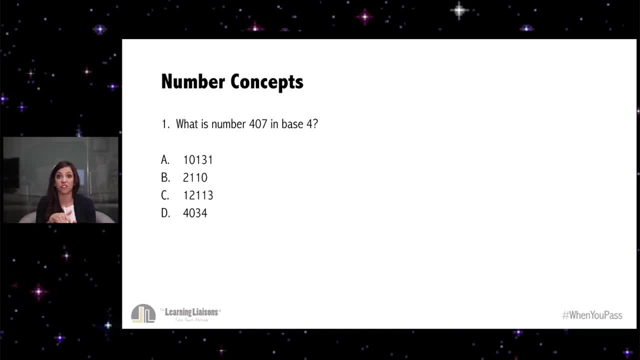 would divide it by 6.. We're dividing by 4 because they're asking for base 4.. And I'm going to start from the bottom of my page and work up and you'll see why in a minute. So 407 divided by 4.. 4 goes into 4 once And I'm going to go through my algorithm. 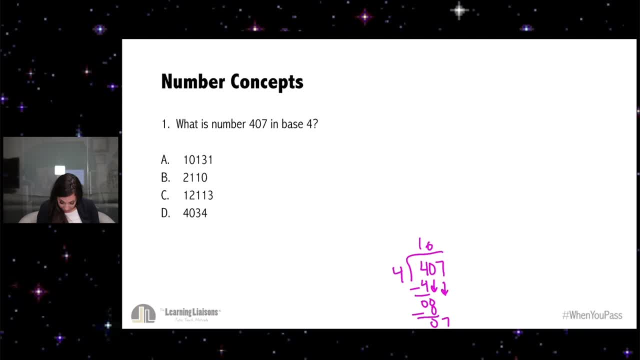 And divide this out, 4 goes into 7. one time You have to represent your remainders. That is extremely important in the representation in base 4, or any base for that matter. So I'm going to have a remainder of 3.. You're not going to do anything with it yet You're. 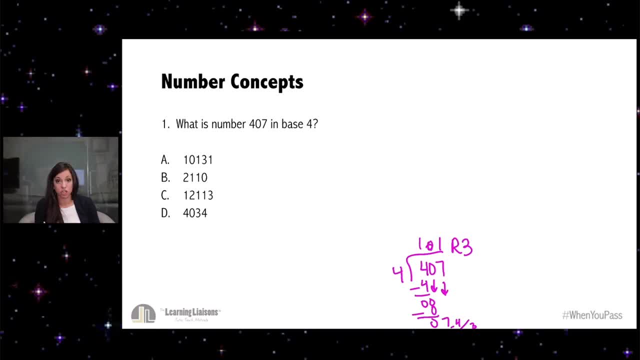 just going to write it Now. I'm going to divide 4 by 101, because that's the number that's on the top. So 101 divided by 4.. And I'm going to go through that same process And I'm going to represent my remainder Now. 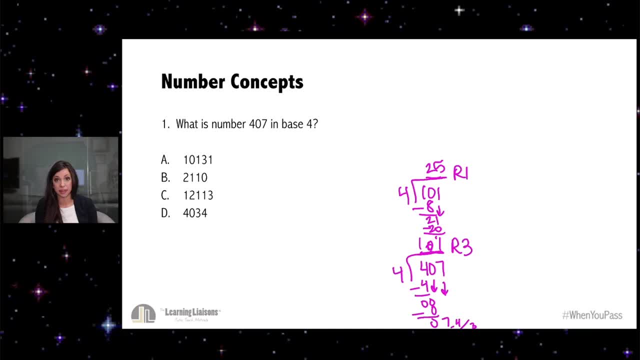 I'm going to divide 4 by 25, because that's the number that's on the top 25 divided by 4.. Represent my remainder again. Now I'm going to divide 4 by the number 6.. Now I have a. 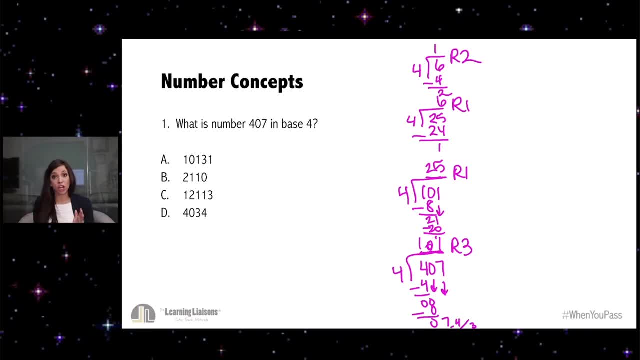 number that can't be divided by 4.. So now I know that in base 4, which is, I divided all of those numbers by 4, I'm going to start at the top right here And I'm going to cycle down And it's going to create my number. So my number in base 4 is going to be 1,, 2,. 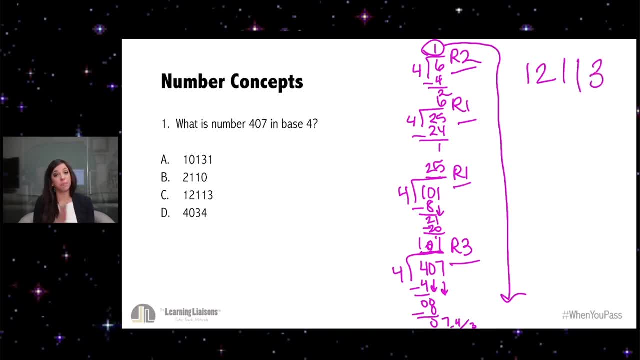 1, 1,, 3.. Because base 4 is a number where we go from the bottom to the top. So I'm going to go up to the number 4. And then we start all over. So it would go 0,, 1,, 2,, 3,, 4.. And 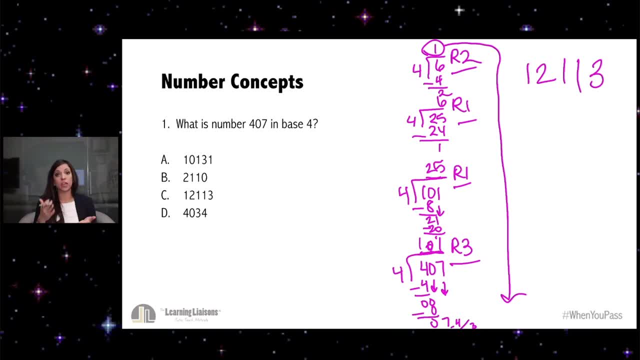 then it starts back over again, Where in our number set we go from 0 to 10. And we start over by adding another 10.. In base 4, we just keep adding extra 4s, Which again it's a. 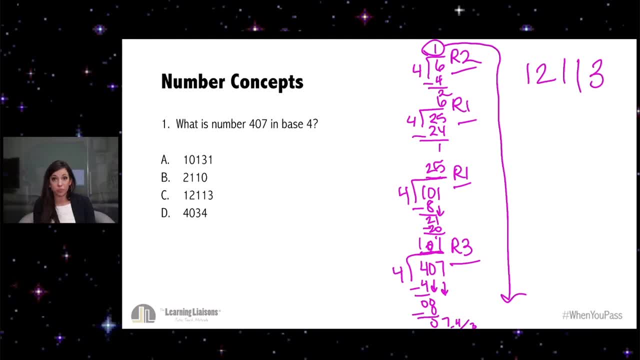 concept that's very abstract for us, But if you can remember this process, you'll be successful on these kinds of problems. So our answer is the letter C: 1, 2, 1, 1, 3.. Remember. 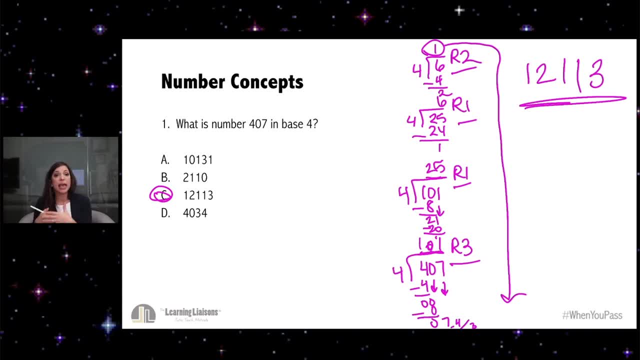 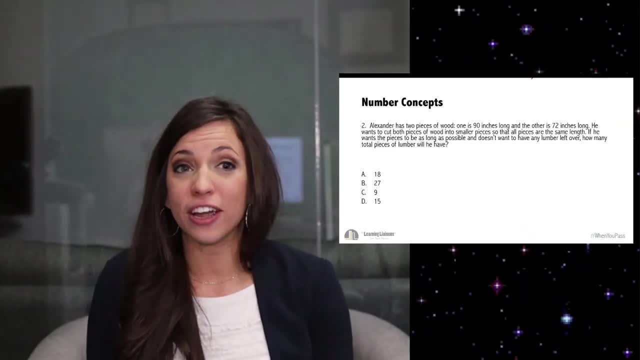 those remainders are super important in finding out what your answer is in a base of any kind of number. Excellent job. Let's move on. Number 2.. Alexander has two pieces of wood. One is 90 inches long And the other is 72 inches long. He wants to cut both pieces of wood. 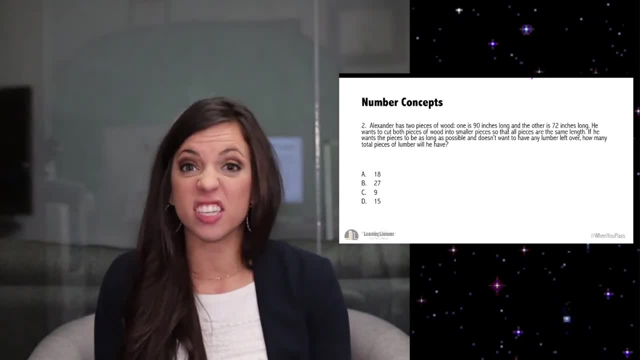 into smaller pieces so that all the pieces are the same length. If he wants the pieces to be as long as possible, then he needs to cut them into smaller pieces. So he's going to stop at the bottom. He's going to leave the rest of the pieces, All right, And he'll. 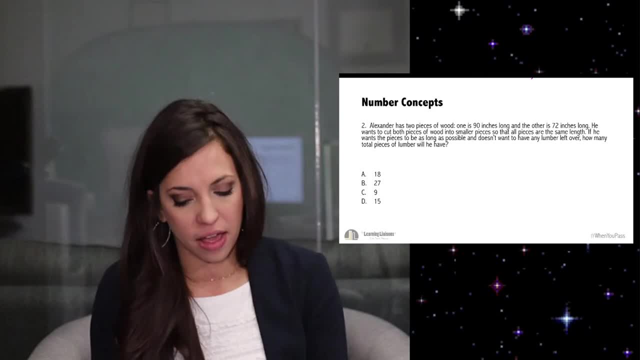 possible and doesn't want to have any lumber leftover. how many total pieces of lumber will he have? A 18,, B 27,, C 9, or D 15.. Go ahead and solve it. You've got 60. 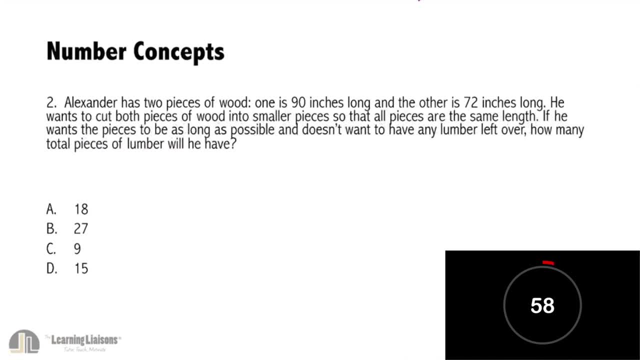 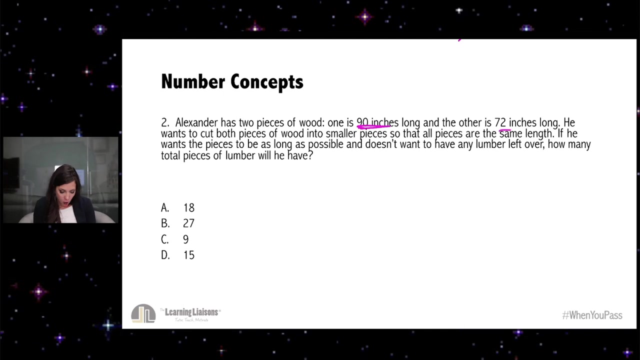 seconds. you All right, We know that he has two pieces of wood, One is 90 inches, One is 72 inches- And he wants to cut those pieces of lumber up. Cut them up, Cut them up. He wants to divide these numbers up, But they all need to be the same length and he doesn't. 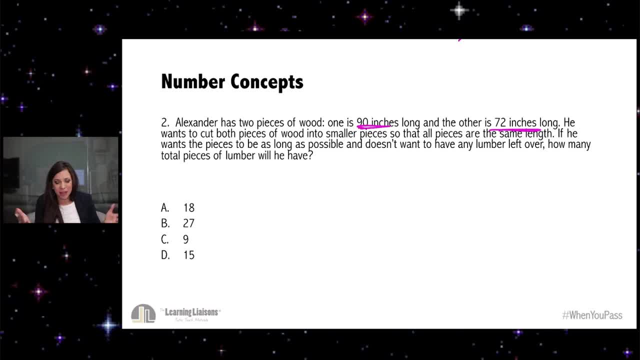 want to have any leftovers, which is remainders when we talk about division. So how many total pieces of lumber will he have In this problem? we're looking for the least common number, We're looking for the greatest common factor, We're not looking for the least common multiple. 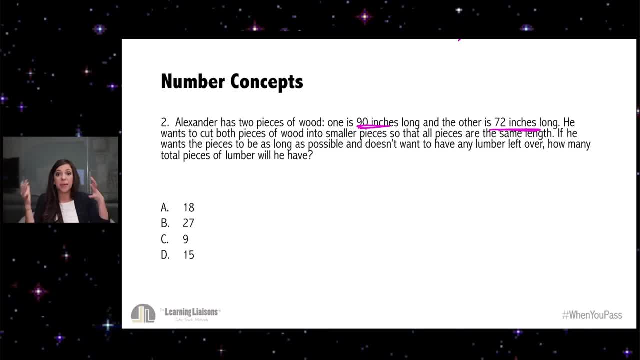 We're looking for the greatest common factor, which is the biggest number that we can have. that multiplies to give us 98. And 72., Because he wants the most amount of pieces without any leftovers. So I'm going to look at these two numbers and I'm going to start listing all of the factors. So we've got 1 in 90,, 2 in 45,, 3 times, 30,, 4 times, nothing, 5 times. And some exams allow you to use a calculator. If you have a calculator, you can use it. 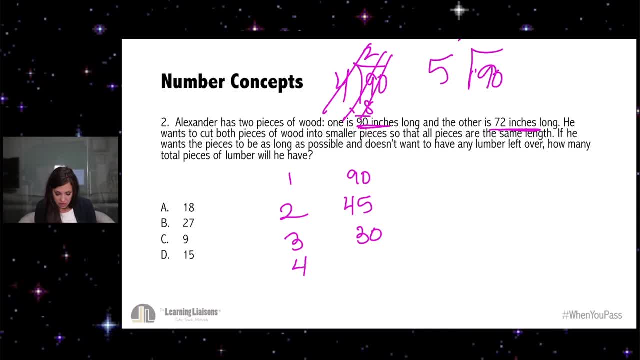 So if you don't have a calculator, this is how you can solve it: 5 times 18.. And we're going to stop there and start listing the factors of 72 and see what we get: 1 in 72,, 2 in 36,, 3 in 24,, 4 in. 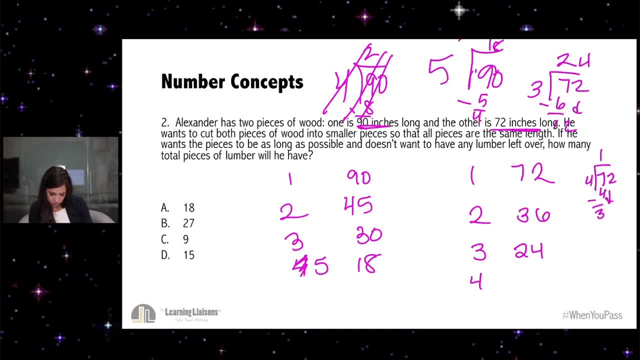 18. 18.. Look at that. We know that 18 and 18 are both multiples of 90 and 72, which means I can divide 90 by 18.. I can divide 72 by 18 and that's the biggest number that each of them have that I can cut those pieces of wood into. 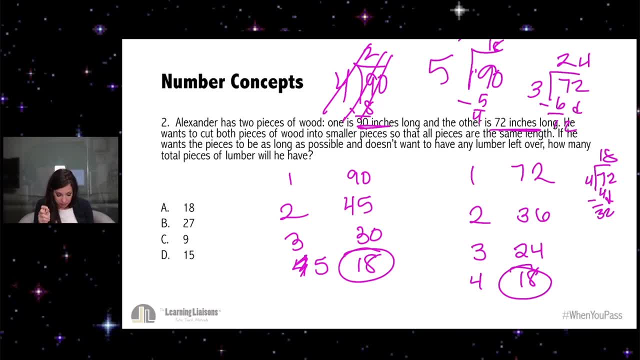 However, the question asks us how many wants us need, since for how many Nats pieces of lumber will he have? not? how big are the pieces? Well, that means that letter A is not correct, because the pieces are each going to be 18 inches long. I'm going to get five pieces. 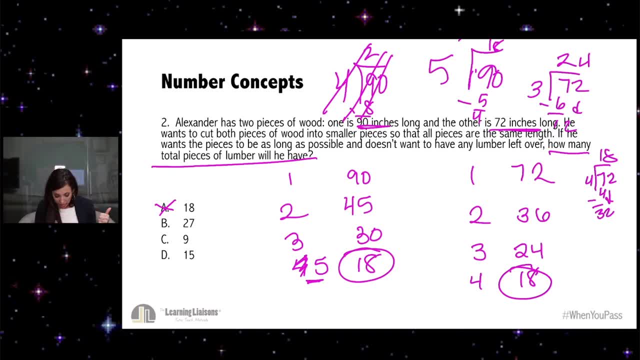 that are 18 inches long out of my 90 inch piece of wood, And I'm going to get four pieces of wood that are 18 inches long out of my 72 inch piece of wood. Five plus four is nine, So I know my. 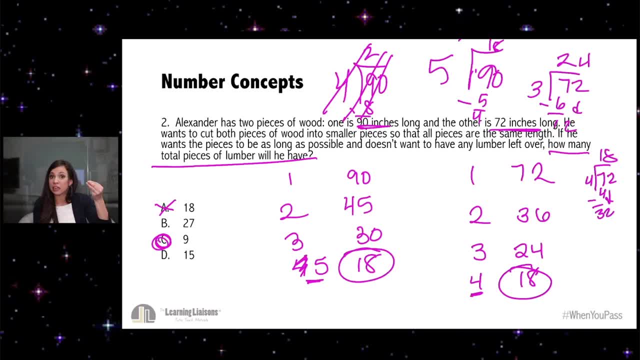 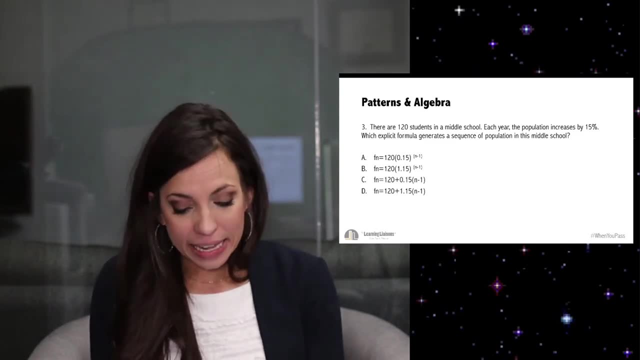 answer is nine, but they threw that 18 in there to trick us, because 18 is actually the greatest common factor. So excellent job working through that problem. Let's go on to problem number three. There are 120 students in a middle school. Each year the population increases by 15%. 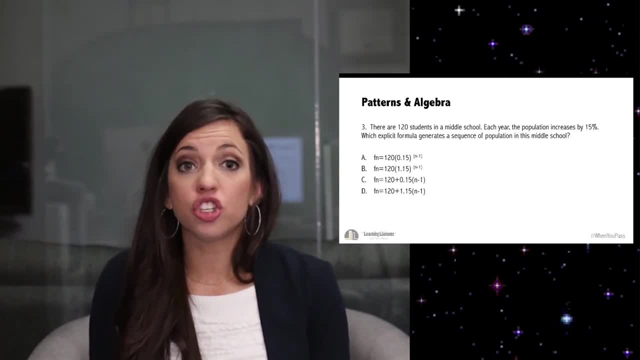 Which explicit formula generates a sequence of population in this middle school. A function equals 120 times 0.15, or 15 hundredths to the n minus one. power B function equals 120 times 1.15 to the n minus one. power C function equals 120 plus 0.15 times. 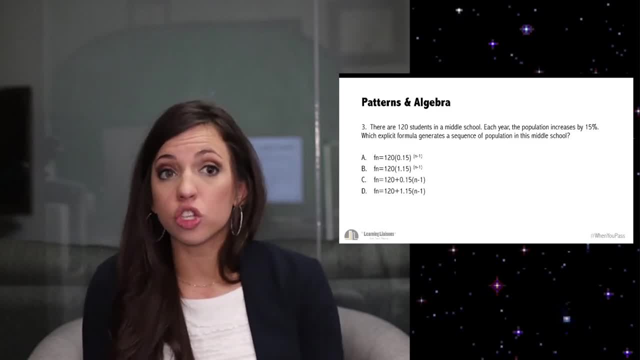 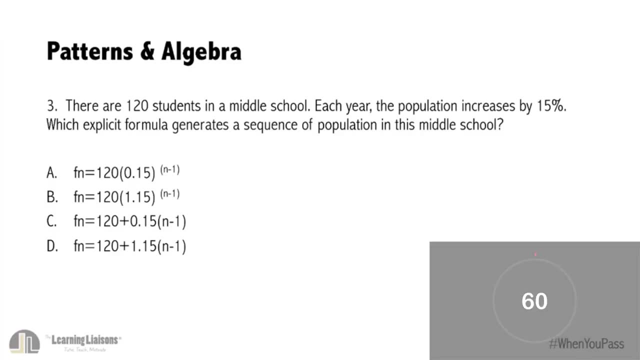 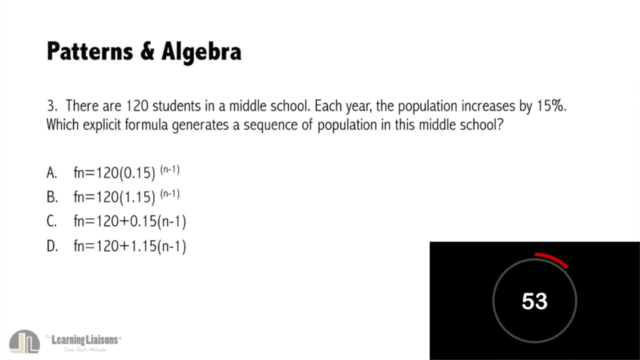 n minus one. D function equals 120 plus 1.15.. C function equals 120 plus 1.15 times n minus one. Go ahead and solve it. C function equals 120 times 1.15 to the n minus one power. D function equals 120 times 1.15 to the n minus one power. 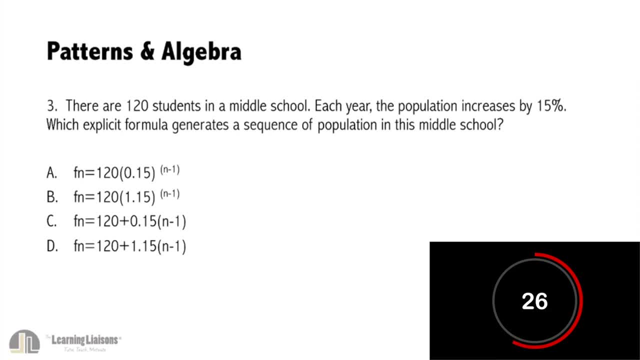 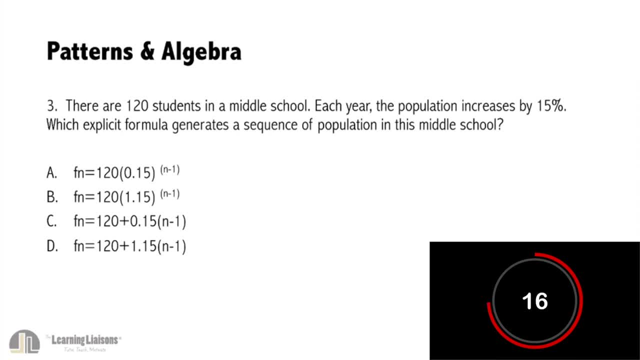 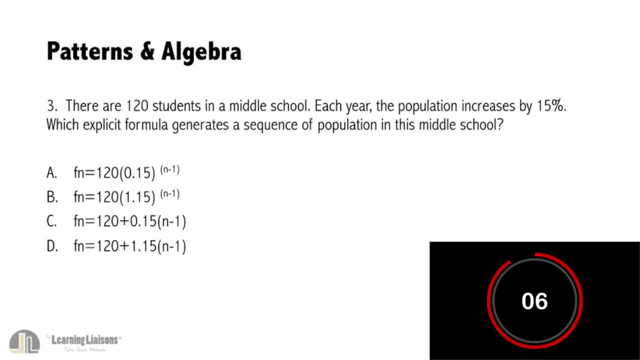 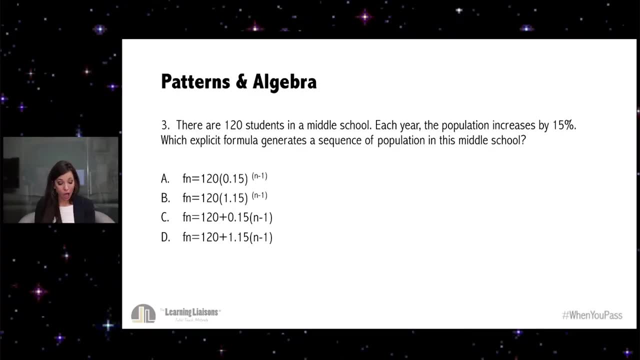 D function equals 120 times 1.15 to the n minus one power. C function equals 120 times 1.15 to the n minus one power. Alright, we know that there's 120 students and our population is increasing by 15%. 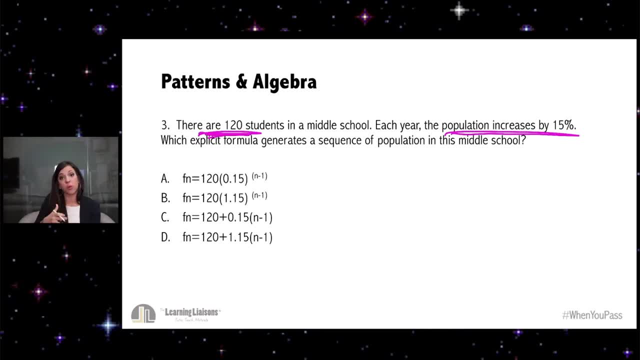 So we know that we're starting with 120 students and we want to find the increase each year. So our formula is going to be our starting number or our starting population. So our formula is going to be our starting number or our starting population. 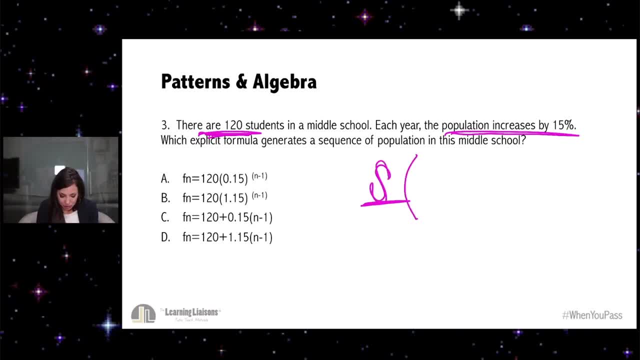 So we'll put an S for start times: our percent to the n minus one power. So we'll put an S for start times, our percent to the n minus one power. N is the number of years that we're looking at. So we know that we're starting with 120, but here's where people make a big mistake. 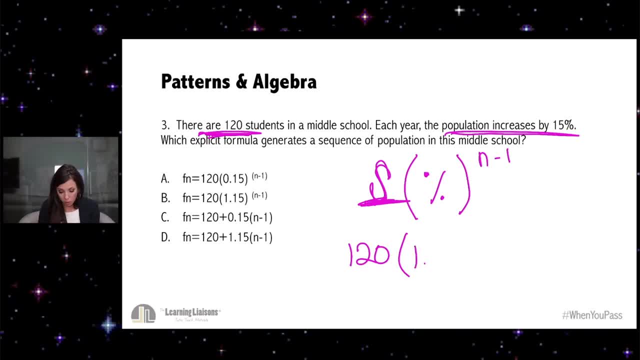 Instead of putting the 1.15, which I'll explain in a minute. most people will just take this percent and throw it in that spot. However, if it's increasing, we want to start with our whole, which is a value of one, and we want to add that percent to that. 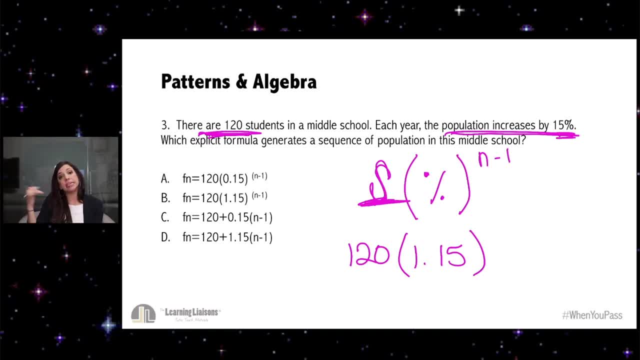 So it's 1.15.. If we're decreasing by 15%, we're going to subtract 15% by a value of one whole, which would give us 0.85.. So if this was a population that was decreasing, our answer would look something like this: 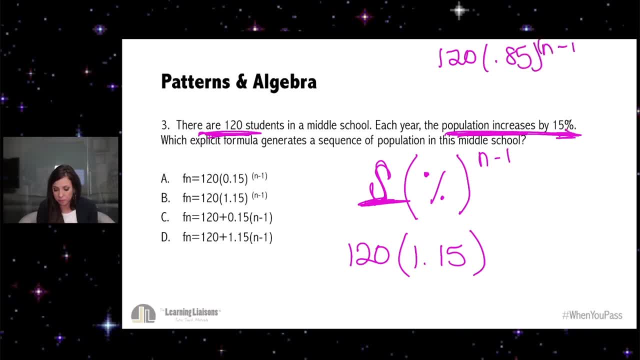 because we would subtract 15%, Because we would subtract 15% from a value of one whole. But because we are increasing, we're going to add 15% to a value of one whole, to the n minus one. N is the number of years, in this case, that we're looking at. 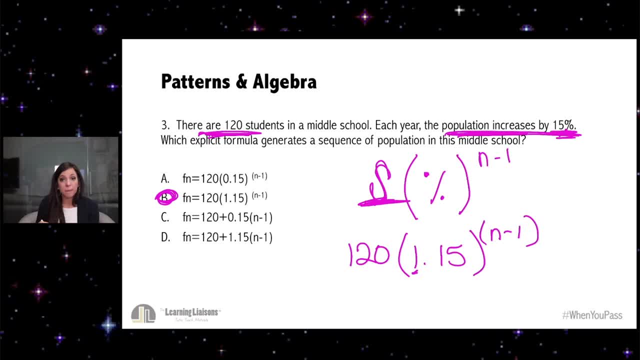 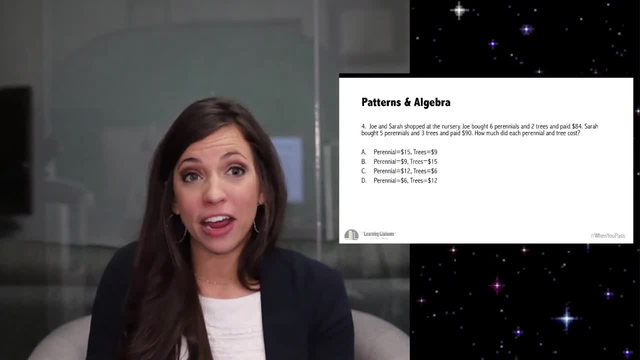 So our answer in this case is going to be B, because we're adding that 15% to the one whole. Excellent job. Let's move on to question number four. Joe and Sarah shopped at the nursery. Joe bought six perennials and two trees and paid $84. Sarah bought five perennials and three trees and paid $90.. How much did each perennial and tree cost? A perennial is $15.. Trees are $9.. B perennials are $9.. Trees are $15.. C perennials are $12.. 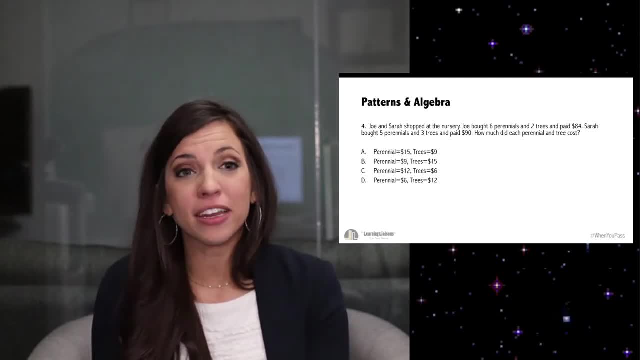 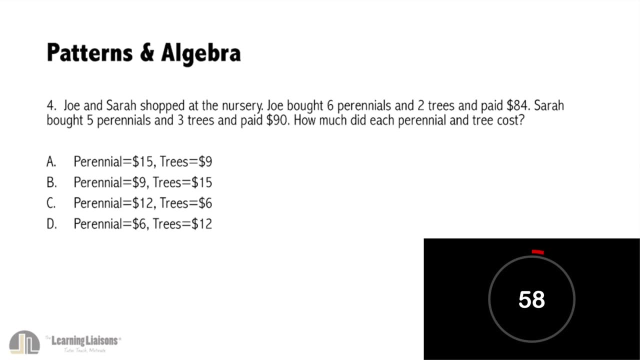 Trees are $6.. Or D perennials are $6.. Trees are $12.. Go ahead and solve it So: you use five perennials and three trees and you get $10.. And there's one perennial And you pay $15.. 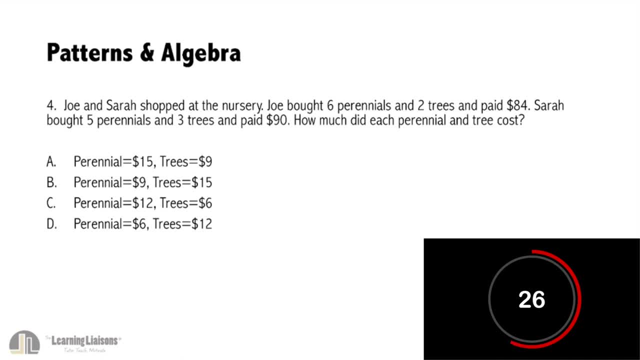 And that's the positive value. What is the negative value of money? Well, you're not going to have to buy 100 perennials. So just look at the picture. So let me show you what that looks like. So what would the negative value be? 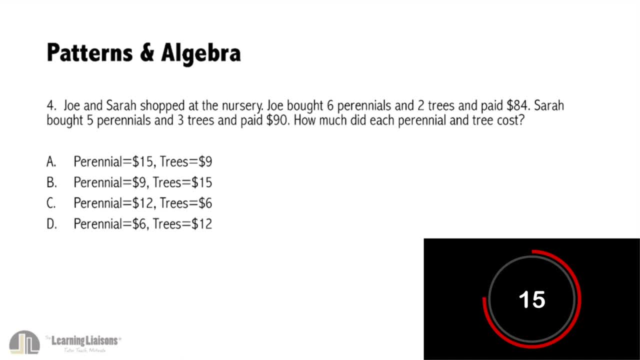 So what I'm going to do is I'm going to say that the negative value is zero, And what I'm going to do is I'm going to add negative value to that. So now you can start looking at the negative value. All right, there's a couple of different ways that we can solve this. 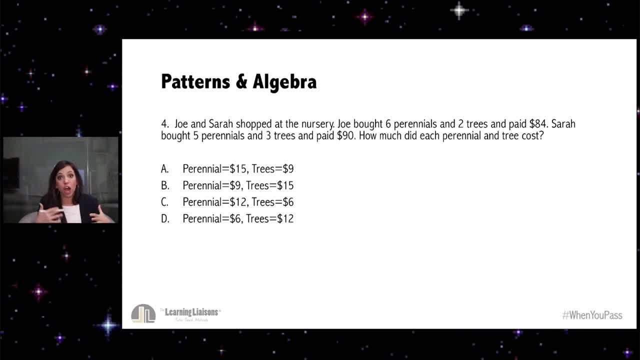 We can use algebra to solve it or we can use our answer choices to benefit us. So we're going to look at both ways to solve it. If we're going to use our answer choices to benefit us, we can literally just take each 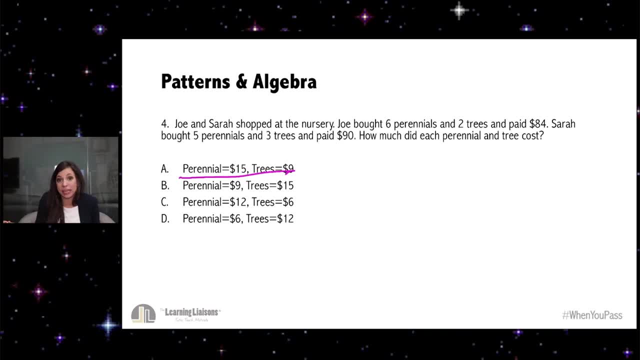 answer choice. plug it into the problem and see what we get. So perennials are $15.. Joe bought six of them. Six times 15 is 90.. Trees are $9.. Nine times two- because he bought two trees- is $18. 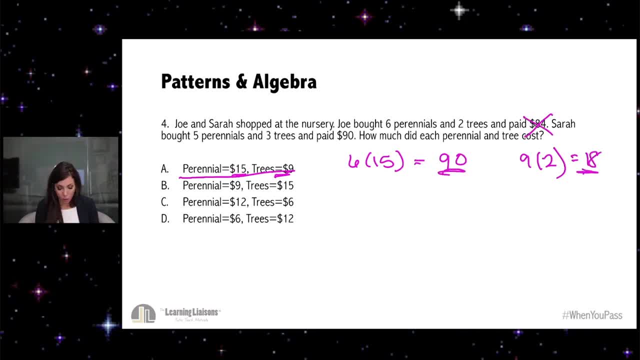 90 plus 18 is not going to be 84. So I know that, But that's not going to be my answer. Letter B: Let's solve that. one Perennial is nine, So six, because Joe bought six perennials. 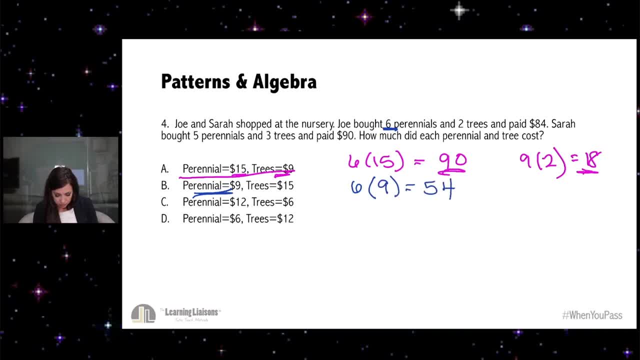 Six times nine equals 54.. And two trees cost $15.. Two times 15 equals 30.. 30 plus 54 is 84.. But I'm not done Now. I have to see if those prices match. Those prices also match Sarah's equation. 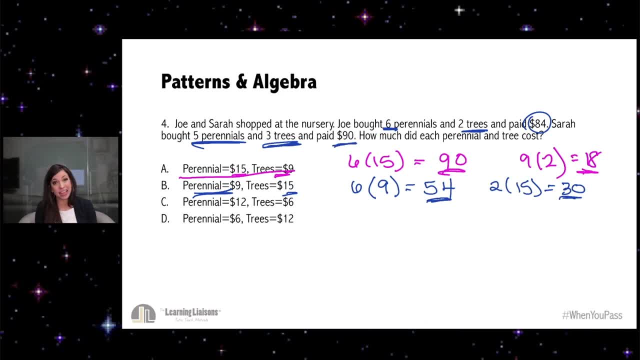 Sarah bought five perennials and three trees and she paid $90.. So let's check it: Five times nine is 45. And three times a value of 15 is 45.. 45 plus 45 is 90. So I've found my answer. 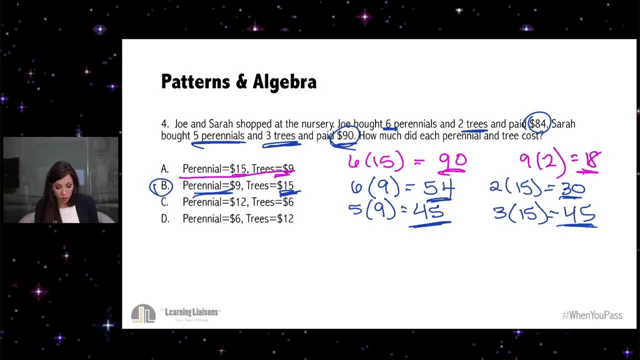 B. But there's also an algebraic way we can solve it as well, Okay, So if I wanted to solve this using algebra, I can use a system of equations. I'm going to define my variables as P equals perennials and T equals trees. 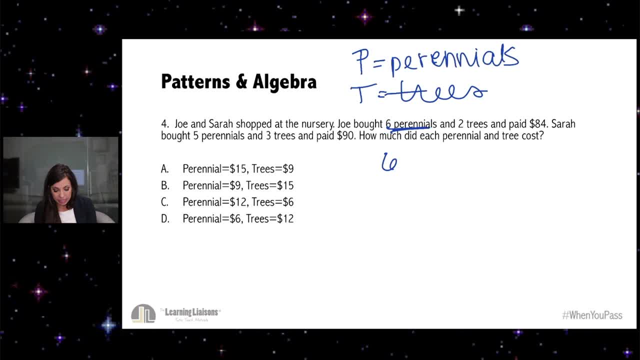 So if he bought six perennials, then he has six P and two trees and he paid $84.. Let's use that same process to figure out the equation for six. So let's take a look at the equation for Sarah. So Sarah bought five perennials and three trees and she paid $90. 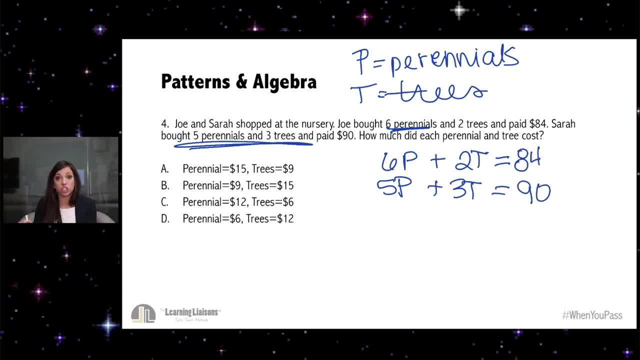 Now I have a system of equations, or two equations, that I can now eliminate a variable to solve. So I'm going to multiply this equation by negative three and I'm going to multiply this equation by two, The entire thing. This equation becomes negative 18 P. 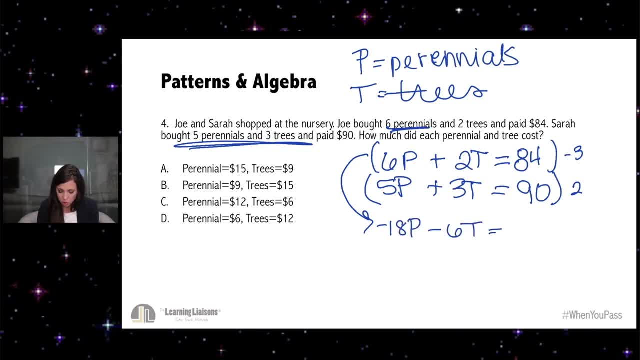 Minus six T equals negative 252.. This equation becomes 10 P plus six T equals 180.. All right, Now I can add my two equations together to see what I get. So negative 18 plus 10 is going to give me eight P. 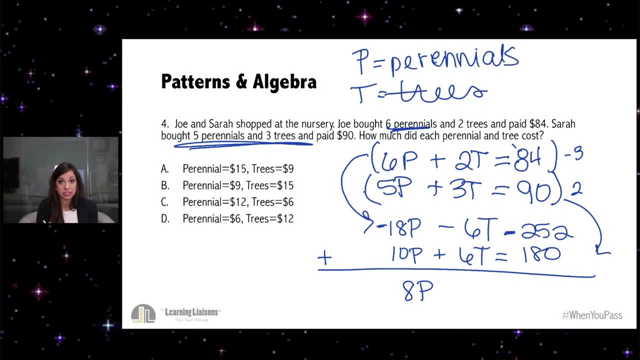 Now you see why I did this: because negative six plus six is zero. That variable crosses out Or eliminates. This is called elimination. with a system of equations Equals, negative 252 plus 180 is going to give me negative 72. Divide both sides by negative eight. 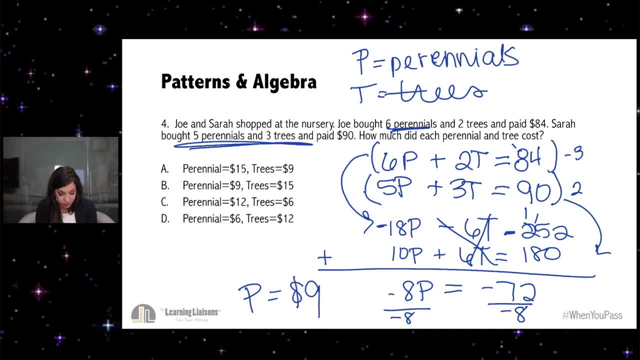 And P is going to equal $9.. So I know that my perennials are $9.. And my trees? if I take this number and I plug it back into an equation, Six times nine plus two T equals 84.. 54 plus two T equals 84.. 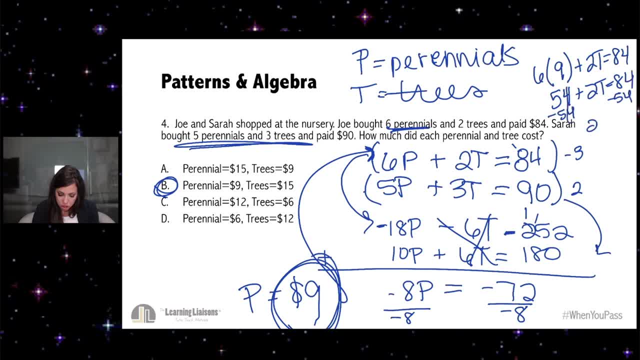 Subtract 54, from both sides, Two T equals 30.. Divide by two T equals 15.. And my trees are $15.. So we can use a system of equations to solve something like this, Or we can just use our answer choices to benefit us. 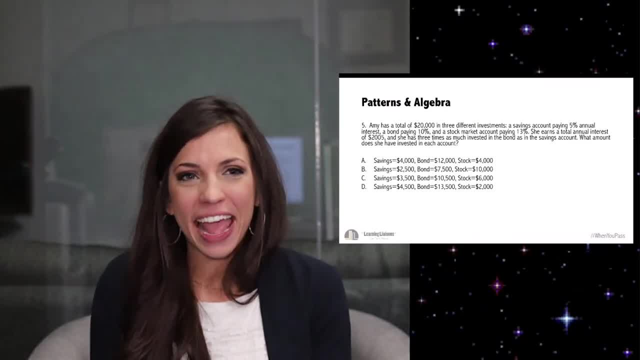 Both ways work Excellent. job Number five: Amy has a total of $20,000 in three different investments: A savings account paying 5% annual interest, A bond paying 10% And a stock market account paying 13%. She earns a total annual interest of $2,005.. 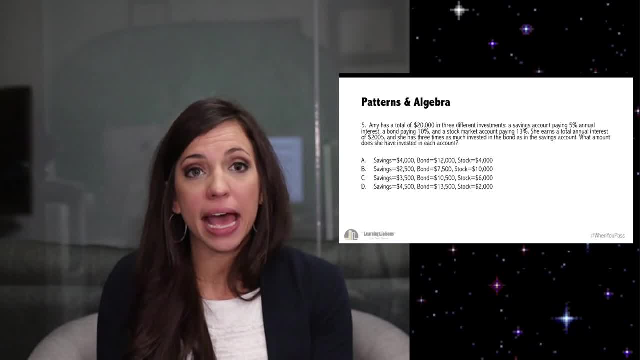 And she has three times as much invested in the bond as in the savings account. What amount does she have invested in each account? A savings- $4,000.. Bond: $12,000.. Stock: $4,000.. B- savings- $2,500. Bond $7,500.. Stock $10,000.. C savings $3,500.. Bond $10,500.. Stock $6,000.. D savings $4,500.. Bond $13,500.. 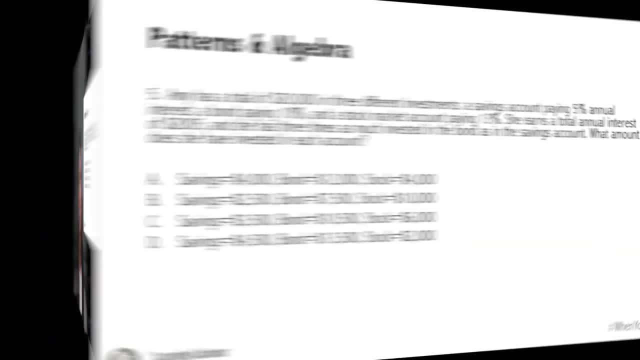 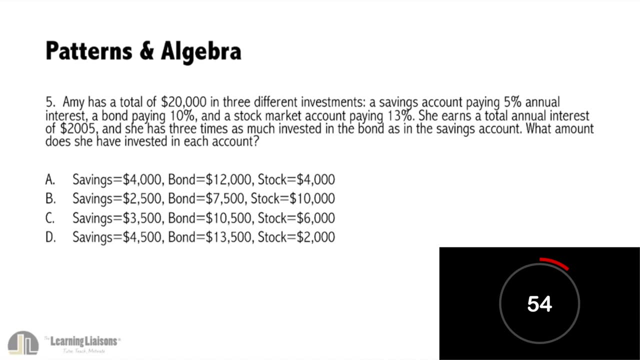 Stock $2,000.. Go ahead and try it. All right, So that's four. That's four of you, And I hope you enjoyed that. Yeah, thanks, It's been wonderful. And thank you, Dave, for being here. 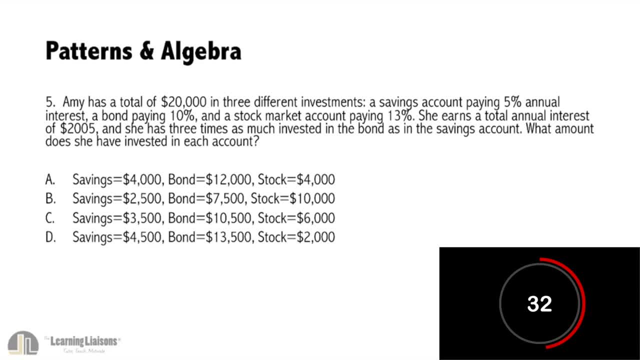 Thank you. Thank you for having me. You're a great person to talk to. Thanks, Dave, Thanks, Thank you. Bye, everybody, and see you next week. Bye-bye, Bye, Bye, Bye, Bye, Bye. 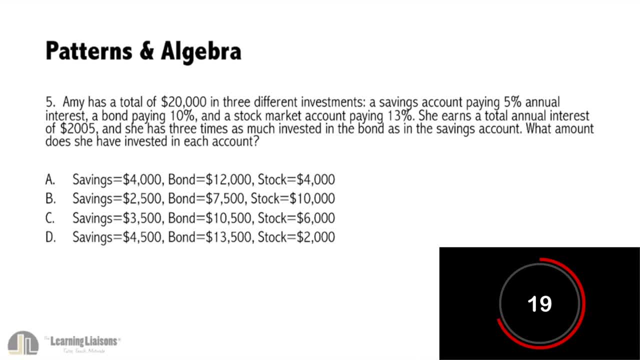 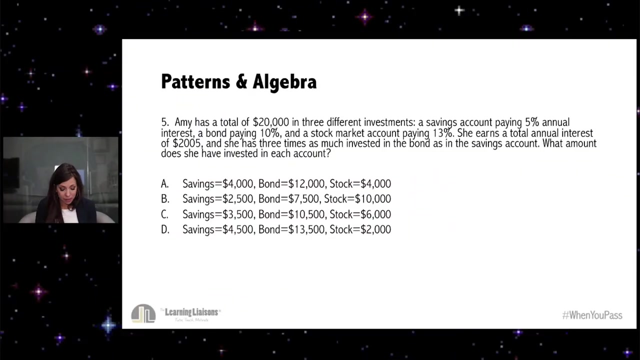 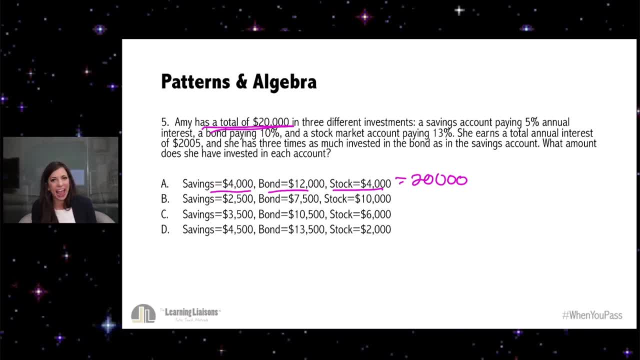 answer choices it does. So we can't eliminate any answer choices based on that, But sometimes you can. So that's going to be the first thing that I do. Then, in this case, I am going to use my answer choices to benefit me. You could use a system of equations to solve this, but because of 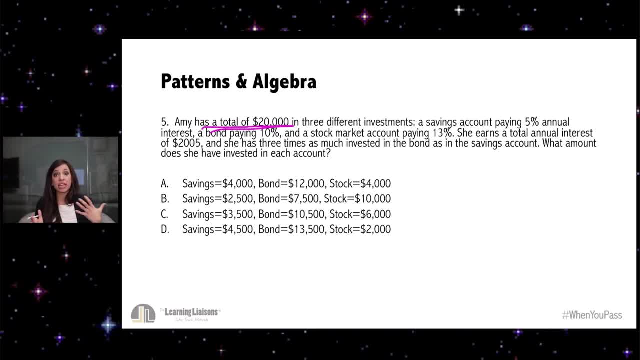 the percent, and it being a three variable equation. it's going to take you a really long time to solve this problem using a system of equations And, let's be honest, we just don't have a whole lot of time to solve these problems, So we're going to use our answer choices to benefit us in this. 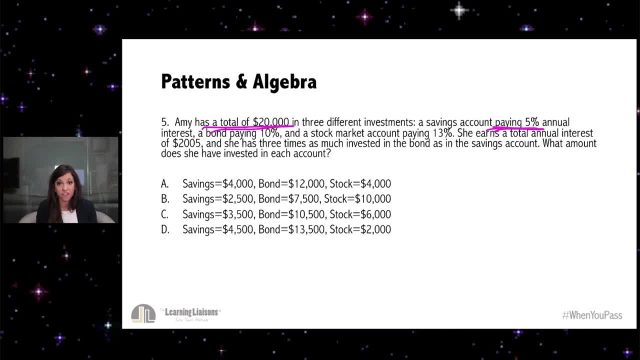 example. So we know we have a savings account paying 5% interest, a bond paying 10% and a stock market account paying 13%. So I'm going to take each answer choice, multiply it by the percentage of interest that we're earning and then add that interest to see if it's $2,005. 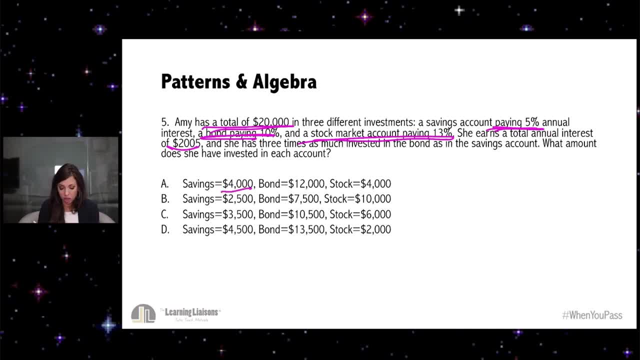 So savings account $4,000.. I'm going to multiply 4,000 times a value of 0.05, because that's how this percent converts into a decimal. I have 5% and I move the decimal over two decimal places. 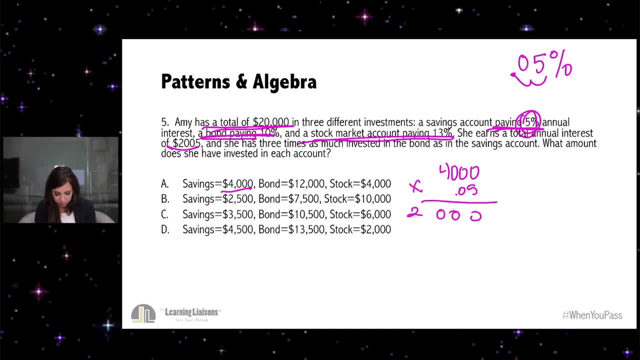 And I end up getting 20,000.. However, I'm going to have to move my decimal place because I was multiplying by a decimal, So I get $200.. And I'm going to go ahead and multiply my $12,000 by a value of 10% and I'm going to move my decimal. 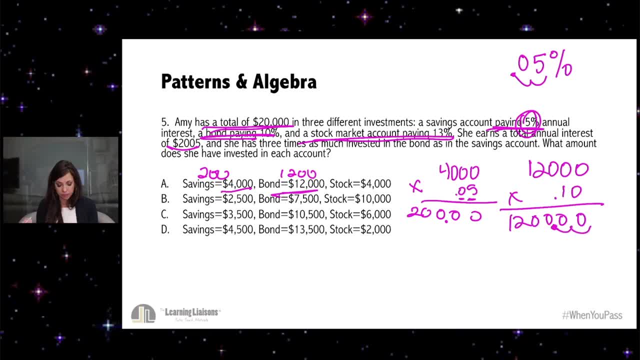 place and I'm going to get a value of $1,200.. Stock: $4,000.. I'm going to multiply that by a value of 13%- 5.. I'm going to move my decimal over two places and I get $520. 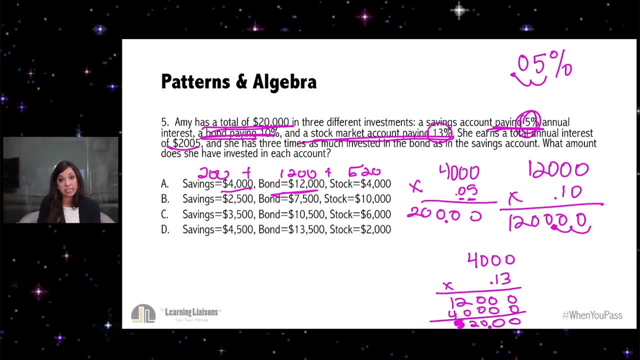 Now I'm going to add those numbers together and see if I get $2,005.. 1200 plus 200 equals 1,400.. 1,400 plus 520 is $1,920.. That is not $2,005.. So I know that answer A is not correct. Let's go ahead and add those numbers together. So I'm going to add those numbers together and see if I get $2,005.. 1,200 plus 200 equals 1,400.. 1,200 plus 520 is $1,920.. That is not $2,005.. So I know that answer A is not correct. 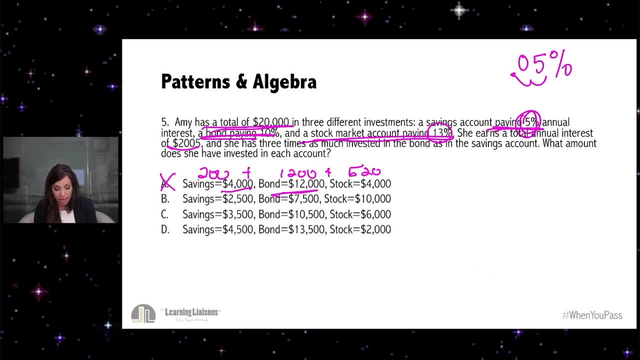 Let's go ahead and move on to answer choice B. Now. some tests allow you to use a calculator on a problem like this. Some do not. If you can use a calculator, well then you can just multiply these in your calculator, which would be awesome. All right, Savings $2,500. 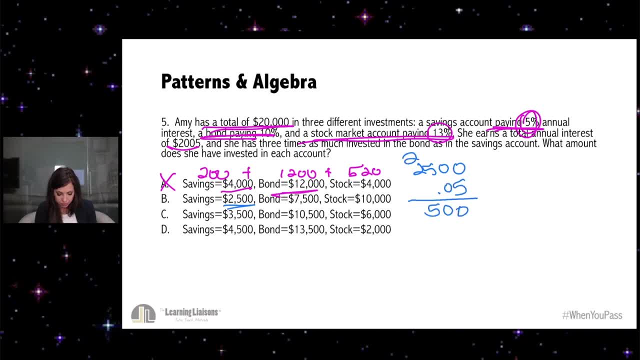 times 5%, I get $125.. Bond: $7,500.. I'm going to multiply that by 10% and move my decimal over to places. I'm going to get 750, so I'm going to add 125 plus 750, plus whatever I get when I multiply. 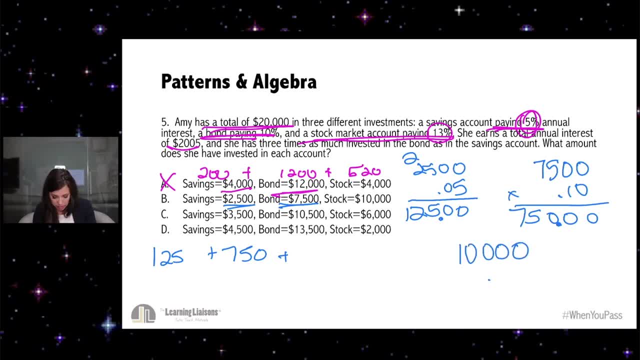 the stock by 13%, 10,000 times 13%. Move it over two places, I get 1,300.. I'm gonna add those numbers together and see if I get 2,005?. I got $2,175.. 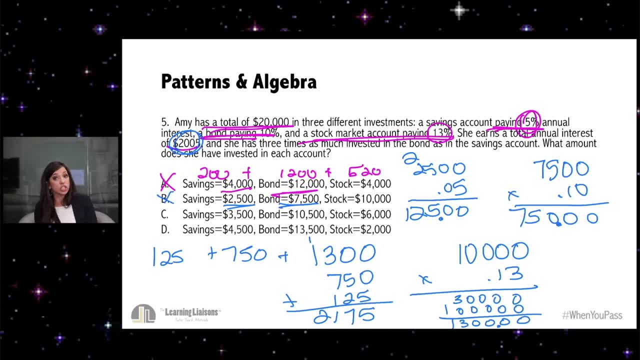 That's not the correct answer either, because, remember, we're looking for an interest value of $2,005.. Let's check out answer number C Going through the same process. So $3,500 times 5%, $175,. plus $10,500 times 10%: $1,050,. plus 6,000 times 13%: $1,050,. plus $1,050, plus 6,000 times 10%: $780.. $780.. I'm gonna add those together and see what value I get.